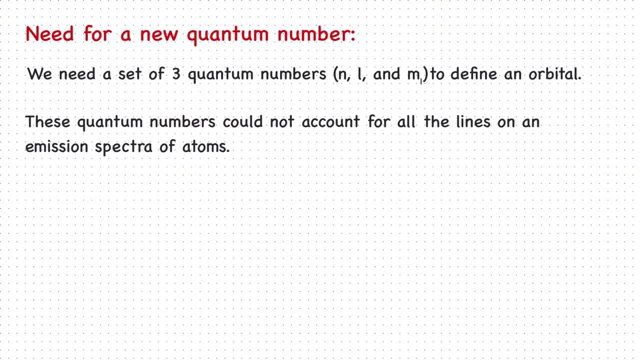 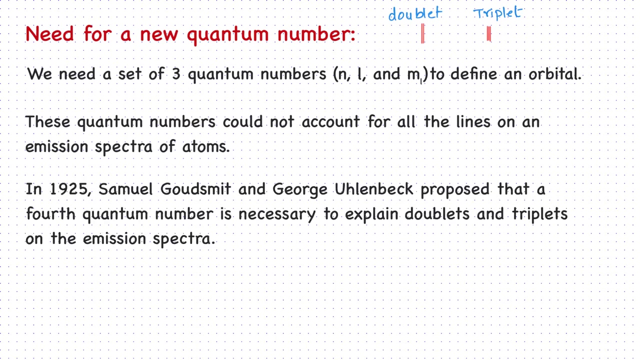 Upon careful observation, scientists noticed that some of the lines on the emission spectrum of certain atoms actually occurs as doublets or triplets, That is, the lines are split into two or three more fine lines In 1925, Samuel Godschmidt and George Ullenberg. 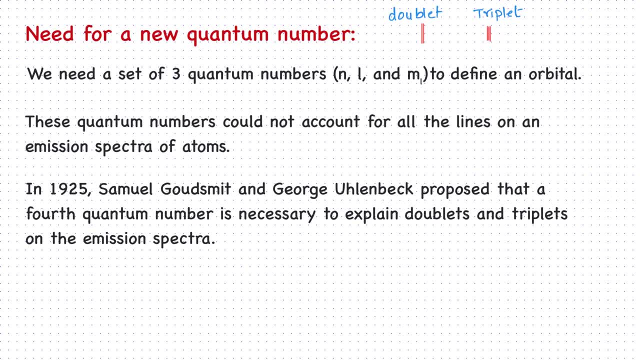 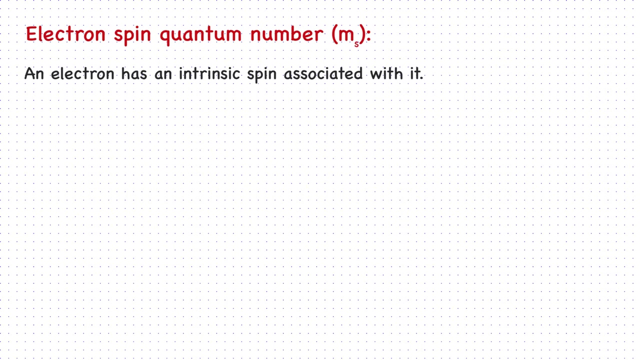 proposed that a fourth quantum number is necessary to explain these doublets and triplets on the emission spectrum. They called this fourth quantum number as the electron spin quantum number, or simply spin quantum number. The spin quantum number is represented by M sub s. According to Godschmidt and Ullenberg, an electron spins around its own axis while randomly moving inside the orbital. 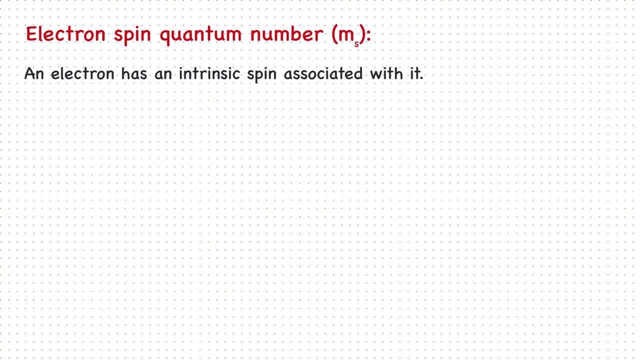 You can imagine that this is similar to the earth spinning around its own axis while revolving around the sun. The electron spin can have two different orientations. For example, the earth can spin in a clockwise or a counterclockwise direction, giving it two different orientations. 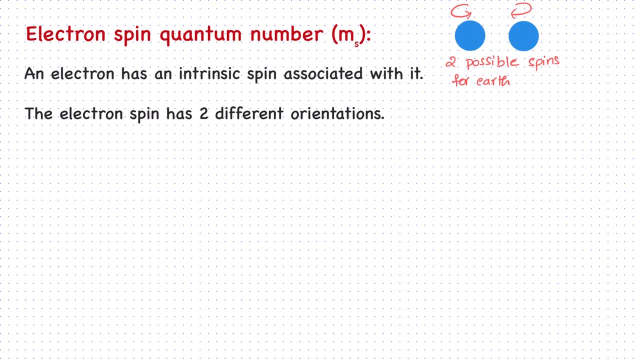 Subatomic particles are a little bit complicated, so therefore we cannot say that the electron can spin in clockwise and counterclockwise direction. but it has two different orientations And the spin quantum number M s is defined to differentiate between these two possible orientations. 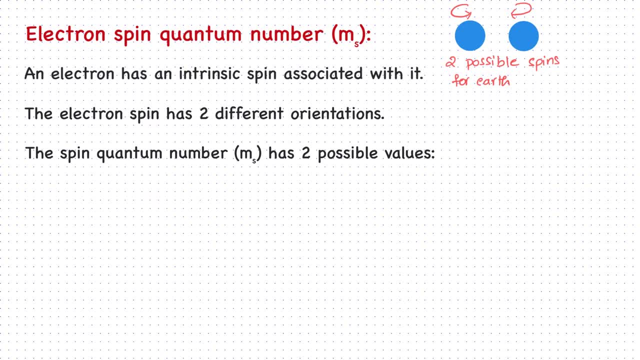 Therefore, the spin quantum number M s has two possible values, plus half and minus half each representing the two different orientations of the electron spin. When we write the electron configurations of various atoms, we represent an orbital by writing a box and an electron by writing an arrow inside the box. 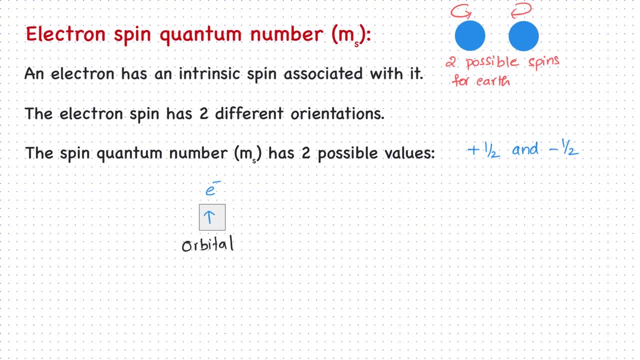 We use an arrow pointing up and arrow pointing down to represent two different orientations of electron spin and therefore the two different spin quantum numbers. It is important to note that the spin quantum number is not a solution for the Schrodinger wave equation. Therefore this is not a property of an orbital. 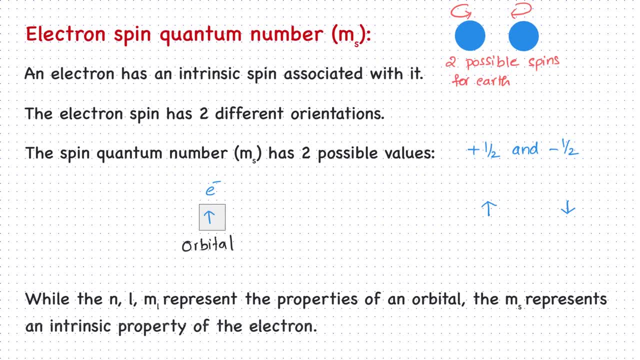 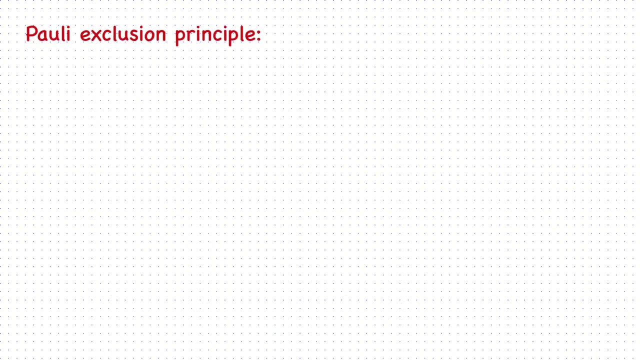 While the principal quantum number- angular momentum quantum number and magnetic quantum number- represent the properties of an orbital, the spin quantum number represents an intrinsic property of the electron. The importance of the electron spin is utilized in Pauli exclusion principle, which talks about the electron occupancy in orbitals. 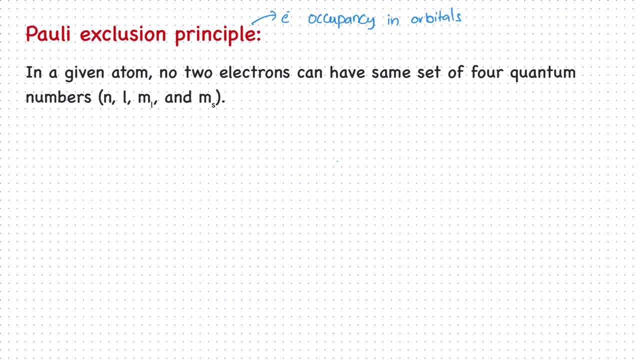 The Pauli exclusion principle states that in a given atom, no two electrons can have the same set of four quantum numbers: n, l, ml and ms. Let us try to understand the implications of this Pauli exclusion principle. Imagine we have an orbital with few electrons in it. 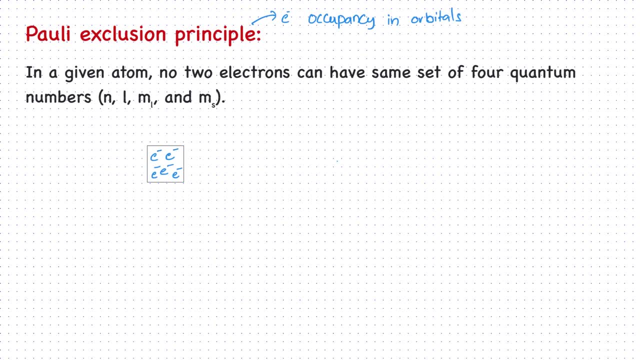 Since these electrons are inside the same orbital, all of them should have same n, l and ml values. Therefore, according to the Pauli exclusion principle, their ms must be different. That means the electron spin associated with all the electrons inside an orbital. 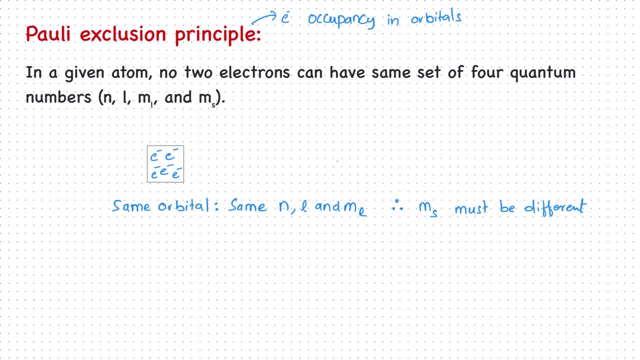 must be different. We learned earlier that there are only two possible values of ms. Therefore we can say that we can place a maximum of two electrons in an orbital, and that too with opposite spins. So as a consequence of the Pauli exclusion principle.